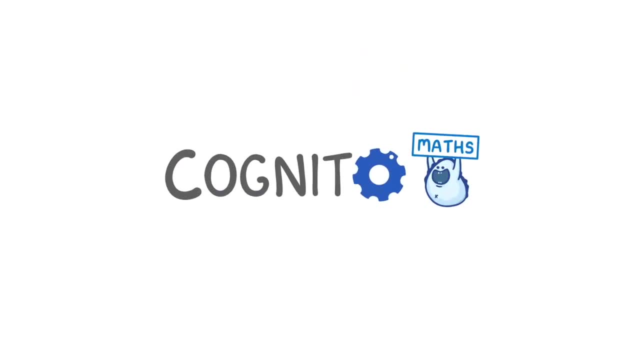 In this video, we're going to quickly run through the names of the eight most common 3D shapes that you need to know, which we also sometimes call solid shapes. First, though, we need to quickly cover how to label the different parts of 3D shapes. If you remember 2D shapes like 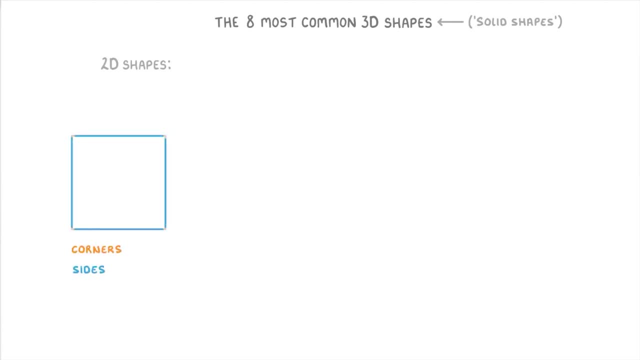 a square, they have corners and sides, But things are a bit different for 3D shapes like this cube. Instead of corners, they have vertices, And if you're just looking at one, we call it a vertex. Then they also have edges, which are these lines in between the vertices. 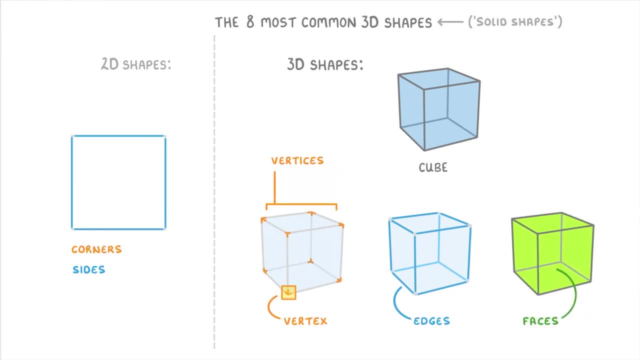 and faces, which are the flat surfaces between the edges. So if we look at our cube, this has a total of 8 vertices, because it has 4 at the top and 4 at the bottom. 12 edges because it has 4 at the top. 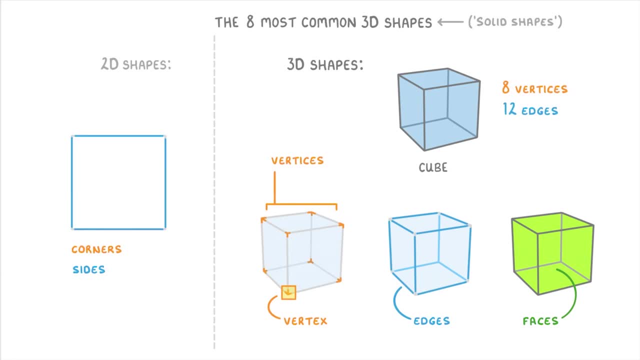 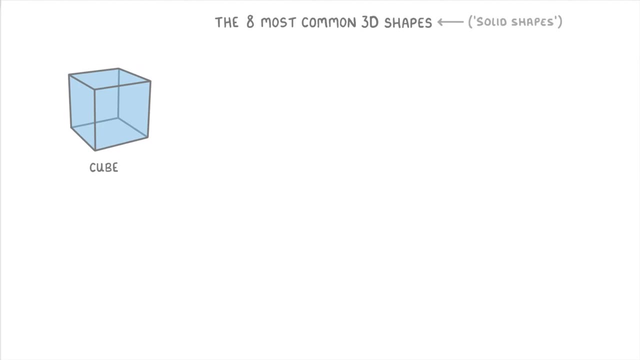 And then we've got 10 edges And then we've got 1 bridge because of the shape of the 4 around the middle and 4 at the bottom, and 6 faces If we move the cube over. the other 3D shapes that you need to know are the cuboid, which. 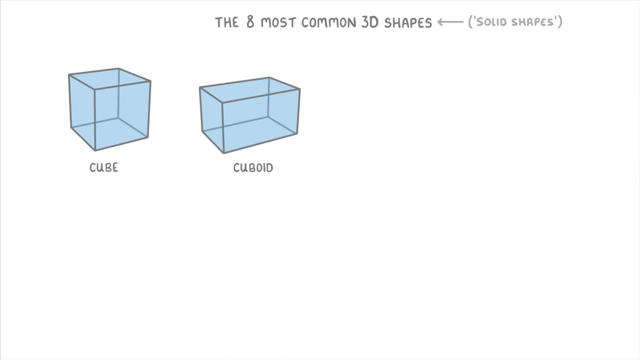 is like a cube, but has been stretched out because it can have rectangular faces rather than all square faces. the triangular prism, which has triangles at either end, connected together by 3 edges, and then the two types of pyramid, which are: the triangle-based pyramid. 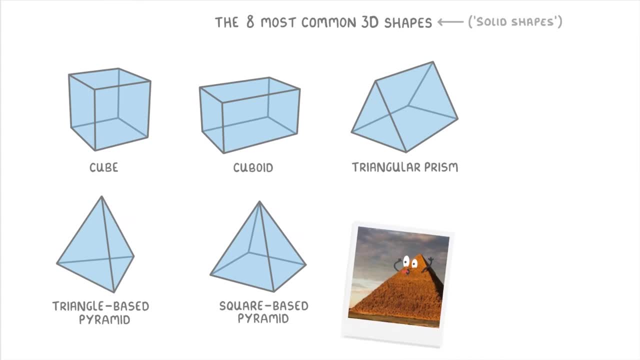 and the square-based pyramid, and they're called this because they both look like pyramids and have either a triangle or a square at the bottom. Also, one thing to point out is you might sometimes hear the triangle-based pyramid being called a regular tetrahedron, but this is just a special case of a triangle-based pyramid. 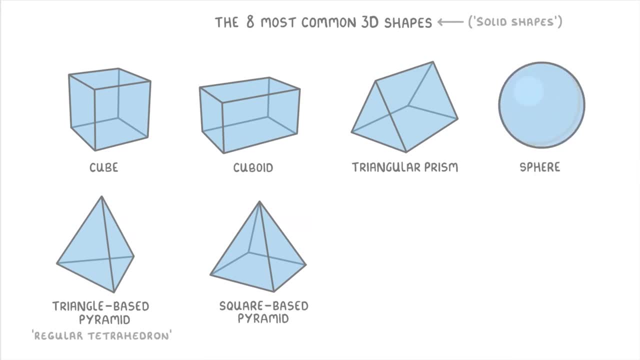 Then the last 3 shapes to know are the sphere, which is like a tennis ball or a football shape, the cylinder, which is like a can of Coca-Cola, and the cone, which is like an upside down ice cream cone. Before we finish, I just want to go through cylinders, spheres and cones in a bit more.